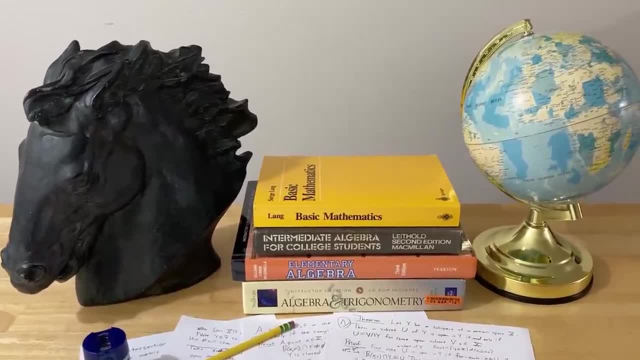 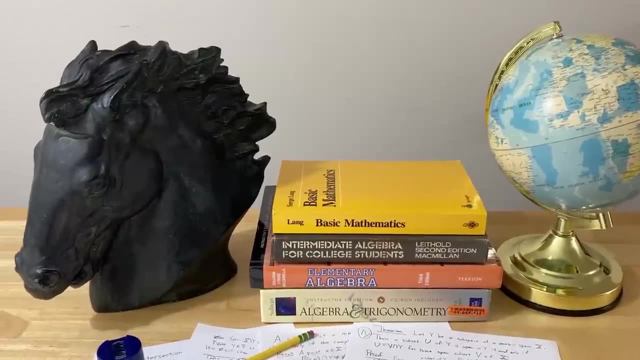 One of the most common questions that people ask is: what is a good book for getting started with mathematics, and the answer is: it really depends on your level of math, But in this video I've picked four books that you can use to get started and chances are if you. 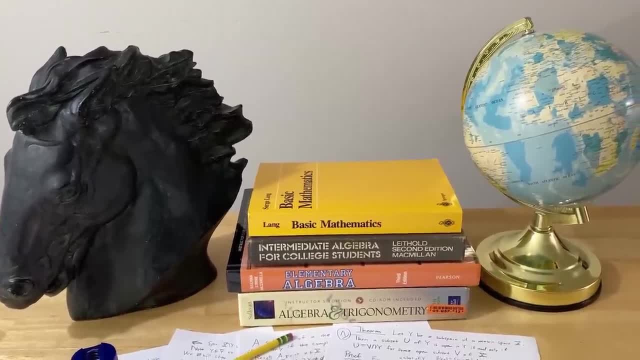 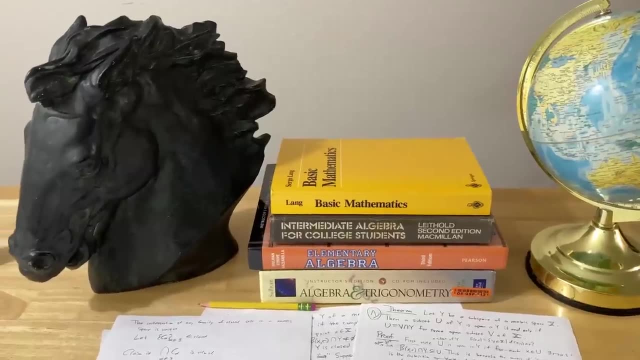 are new to math or you're coming back to math, one of these books will help you, Even if you already know some math. chances are these books will help you because there is so much math in each of these books. Okay, let's go ahead and go through each of these books briefly. 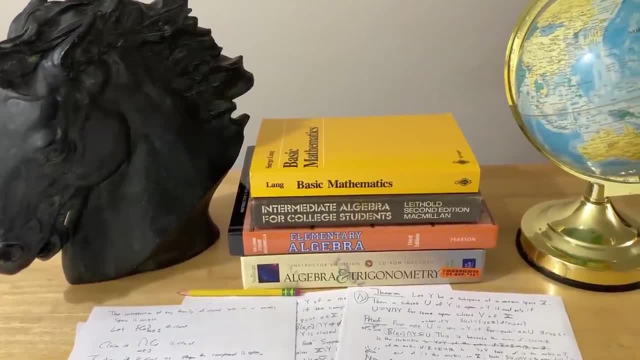 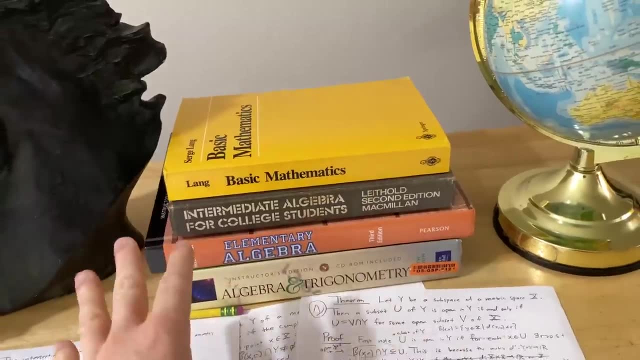 and at the very end of this video, I will tell you which one I think is the one worth buying. Obviously, I bought all four, so I think they're all worth buying. however, if I had to pick one, I think one of these really stands out from the rest. The first book I want to 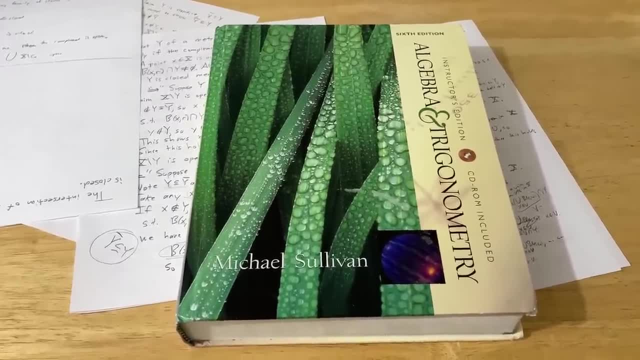 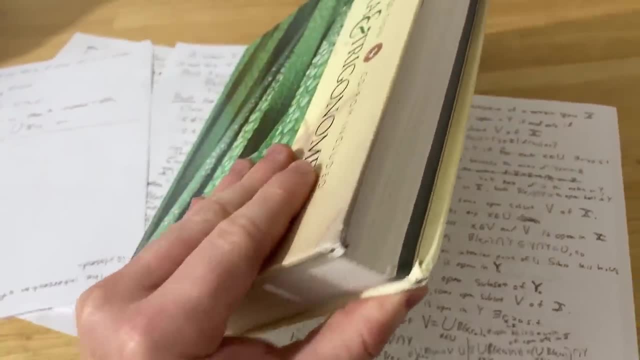 show you is called Algebra and Trigonometry and it was written by Michael Sullivan, So this is a book that you would use if you went to college and took a course perhaps by the name of precalculus or maybe trigonometry, or maybe a precalc trig combo course. 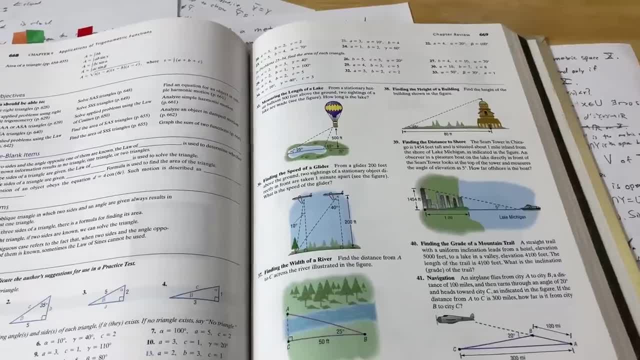 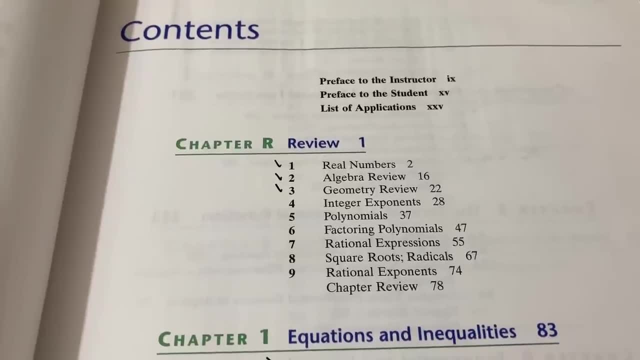 All of those courses would use a book like this. The material in a book like this is usually considered a prerequisite before studying calculus at the college level. Let's briefly go over the contents So you can see what this covers. So chapter R is the review chapter. 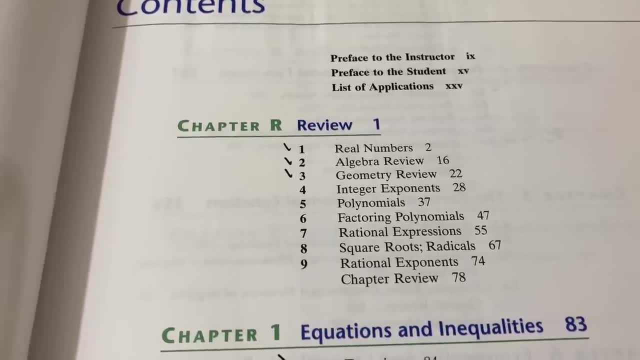 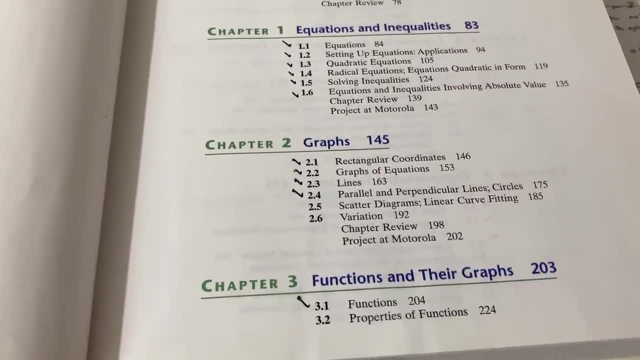 and it basically covers stuff that you might cover in, say, an intermediate algebra course in college. Chapter 1 is on equations and inequalities, 2 is on graphs and 3 is on functions and their graphs. 4 is on polynomial and rational functions, 5 is on the zeros. 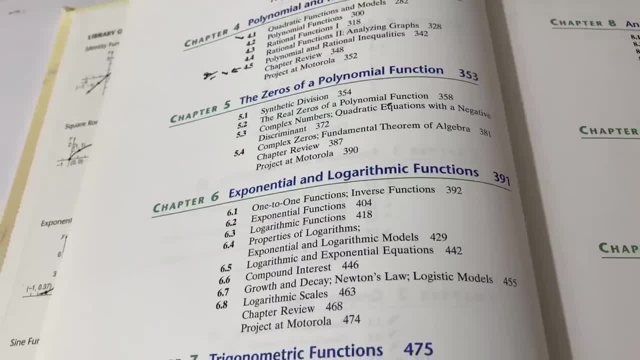 of equations and their graphs. 4 is on polynomial and rational functions. 5 is on the zeros of a polynomial function. Then we have exponential and logarithmic functions. So the first 6 chapters are pretty much what you would study in a college algebra course, although it is missing. 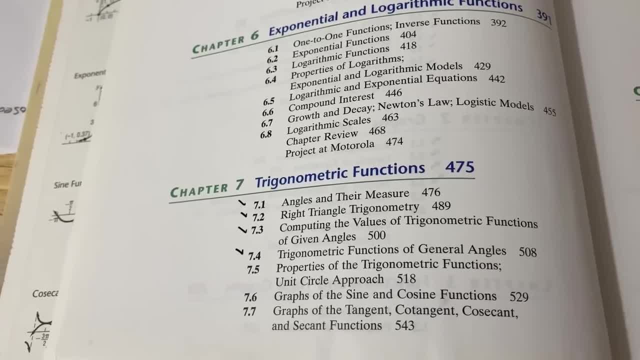 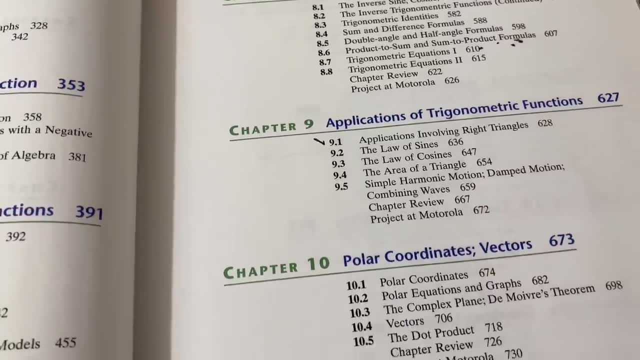 some topics which are covered in later chapters. Chapter 7 is where the trigonometry starts, and then it goes into chapter 8, which is more trig. 9 is more trig and then 10. you talk about polar coordinates and vectors, also usually covered in a trig class. Chapter 11: 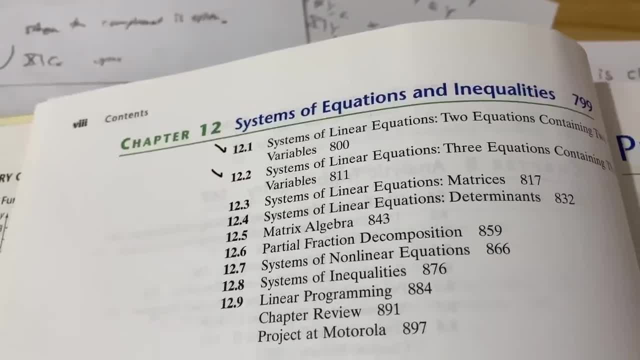 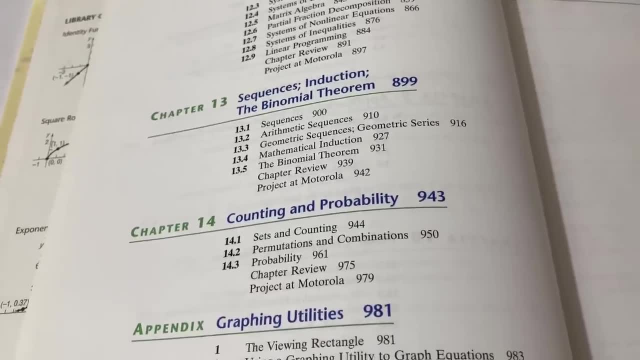 covers conics, which are usually covered in a precalculus class. Chapter 12 is on systems of equations and inequalities, and then it goes on to sequences, induction and the binomial theorem, and then we have some counting and probability and then there's an appendix. So this book contains: 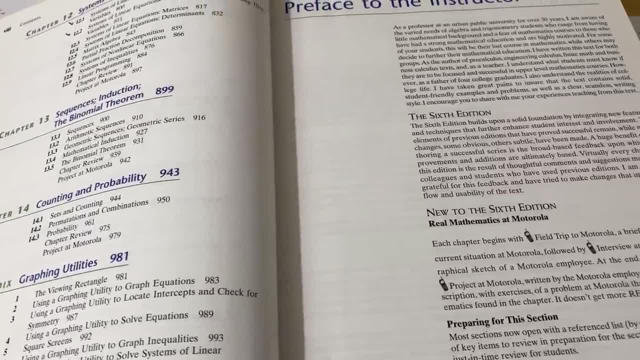 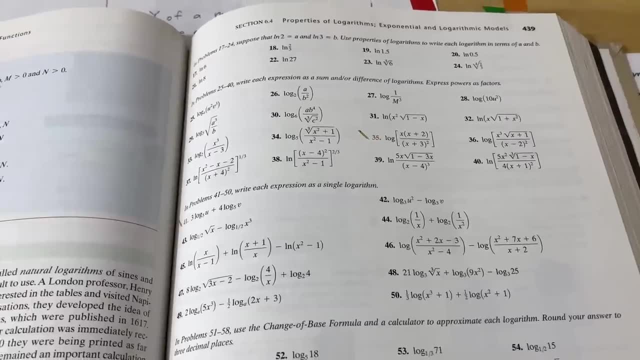 tons of mathematics and it can be used to take various courses in college, either college algebra, precalculus, trig or any combination of those courses. This book has tons of exercises that you can do for practice, and it includes answers to all of the odd-numbered exercises. 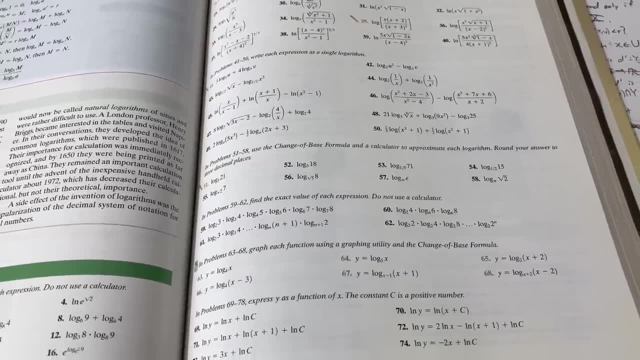 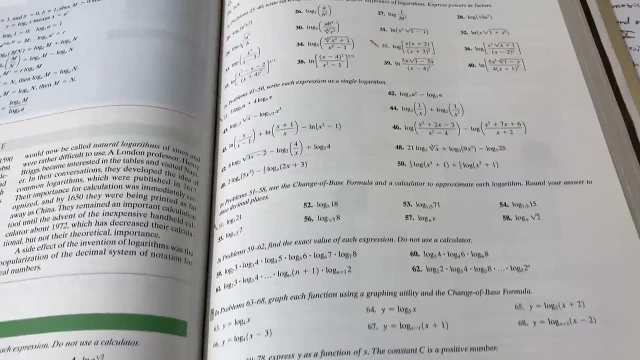 My copy is the instructor's edition, so it does have answers to all of the exercises, But if you get the regular edition, I'm pretty sure you only get the odd answers, which in my opinion is still pretty good, considering how many problems you have in each section. 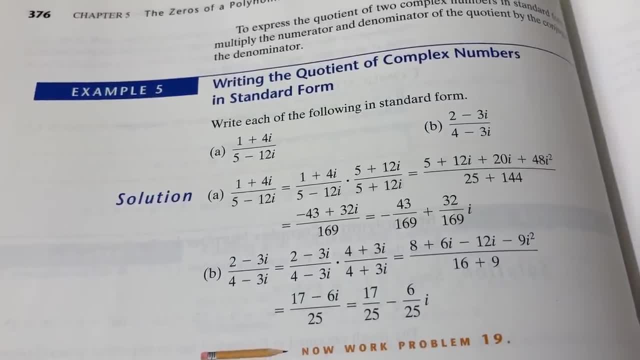 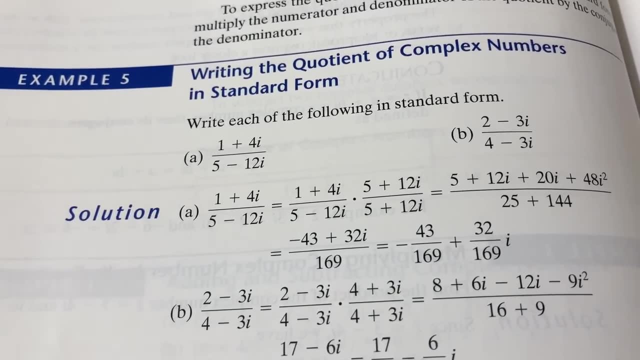 for practice. The examples are really good, as you can see here. they show all of the steps. They're trying to take a complex number and write it in standard form, so they basically multiply the numerator and denominator by the conjugate of 5 minus 12i, which is 5 plus. 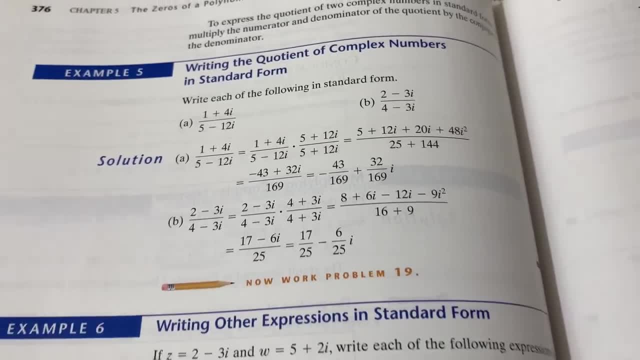 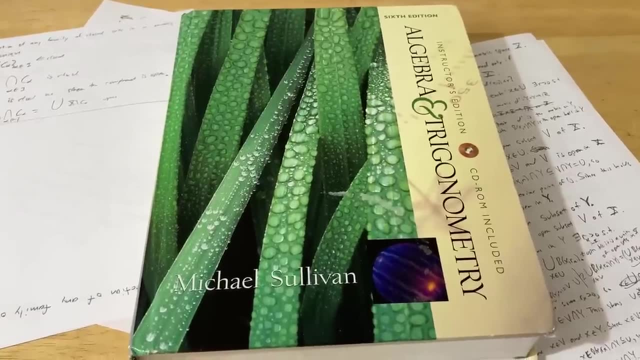 12i and you can see all of the steps are shown. So this is a good book for self-study and it's a good book to use as a supplement if you're interested in learning more about the exercises. Overall, the pros of this book are that it's got tons of problems, tons of information. 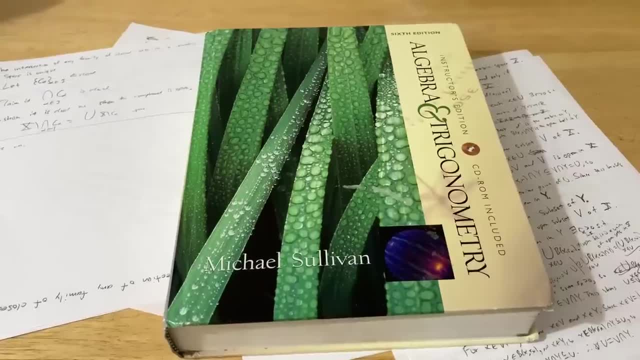 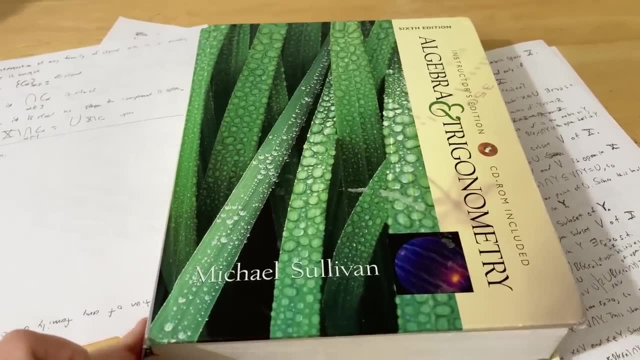 and great examples. Cons: I can't really think of any. This book is going to cost some money. it's not super inexpensive but it is available. You can find it and I'll try to leave a link in the description after I make this video. 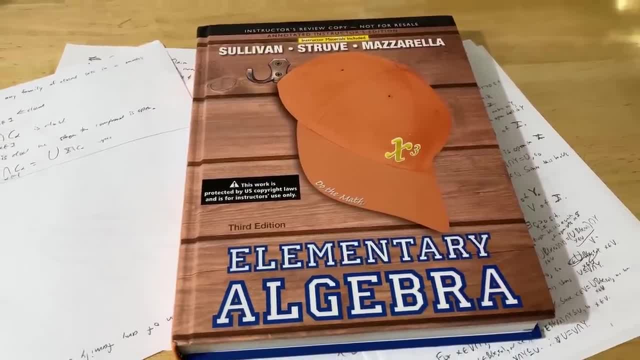 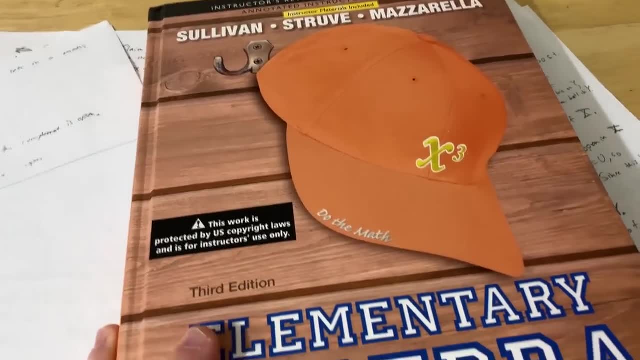 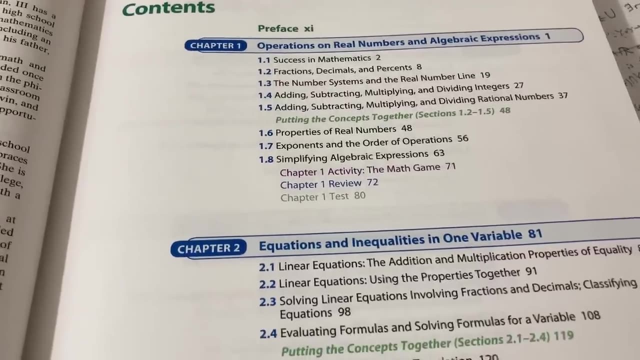 This next book is even more basic. It's called Elementary Algebra, so this is good for someone who is not even ready to take a course like college algebra. yet This is the instructor's edition and this one was written by someone, So this book covers really basic algebra. This is the type of algebra that is covered. 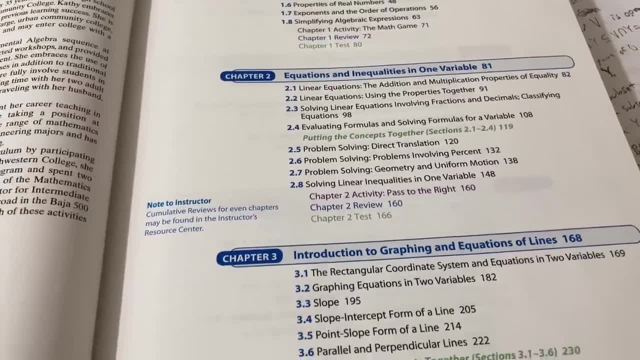 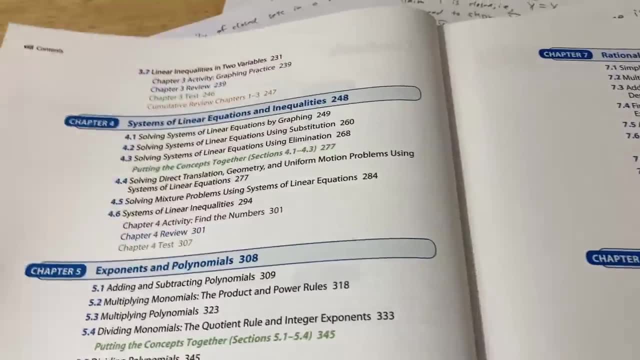 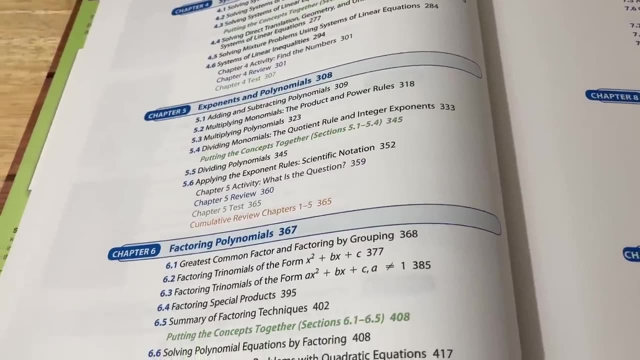 before taking a course like college algebra, usually in a course like intermediate algebra in college. It's very, very basic and I think this is a good book for someone who has really bad algebra skills. so if you're trying to get started with algebra like factoring and 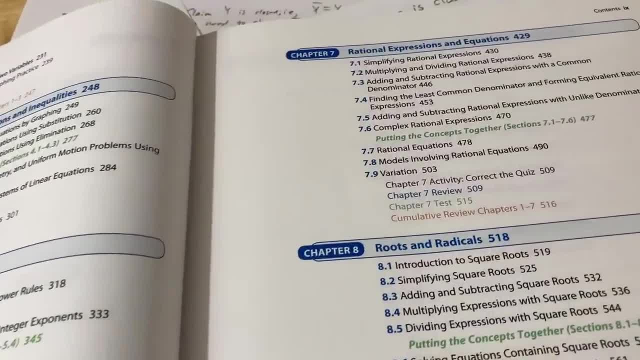 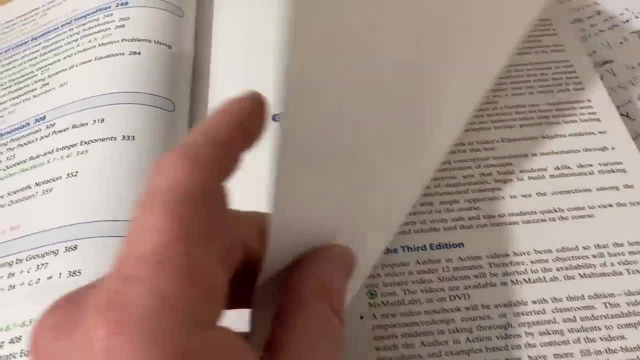 multiplying, just really basic stuff. this is the kind of book that you want. If you feel like you already know how to use the quadratic formula, you already can factor, you already know basic math, then you want to get another book, perhaps like the one 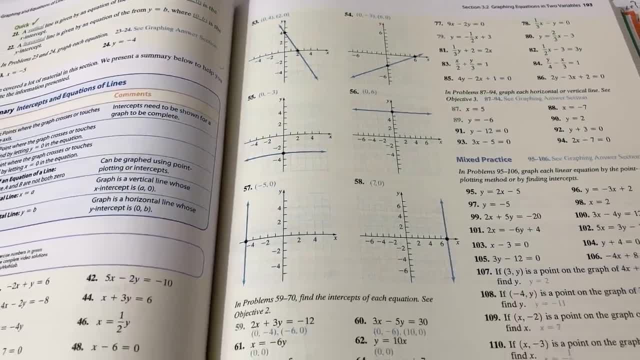 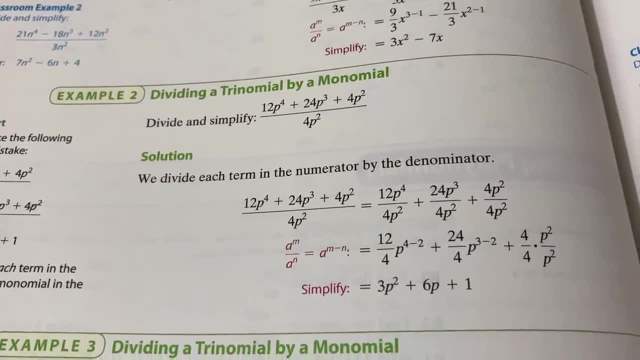 I showed you before. This book also has tons of exercises and you should have answers to all of the odd-numbered problems in the back of the book. Here's a simple example where they divide a trinomial by a monomial, and you can see. 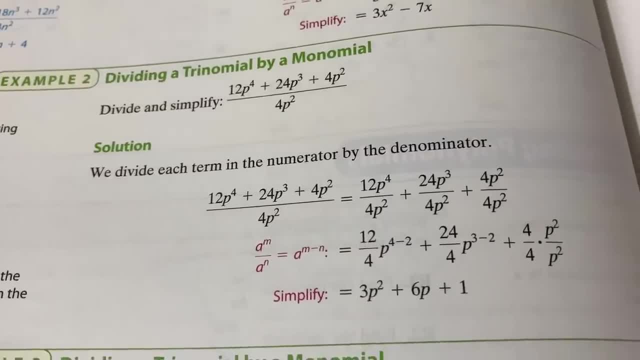 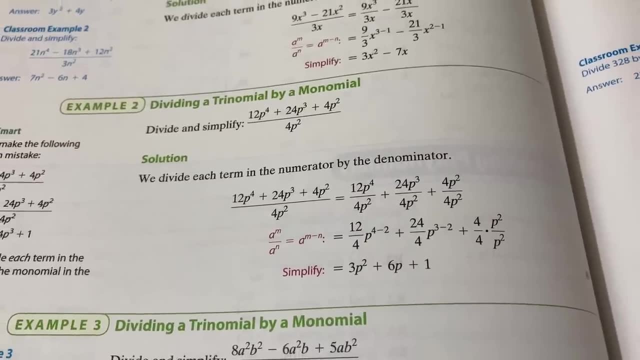 they show all of the steps and they explain the property of exponents that they're using in all of the steps. So I think this is a great book for beginners who want to learn math on their own, great for self-study and also great as a supplement. 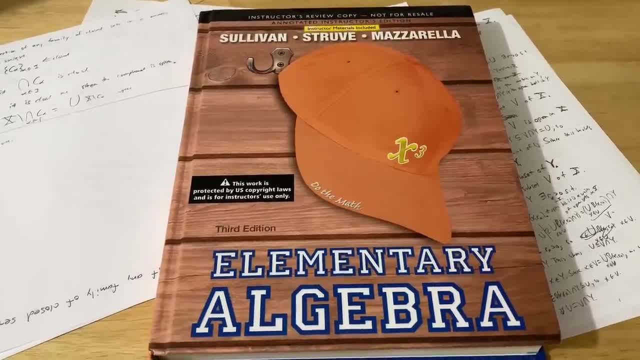 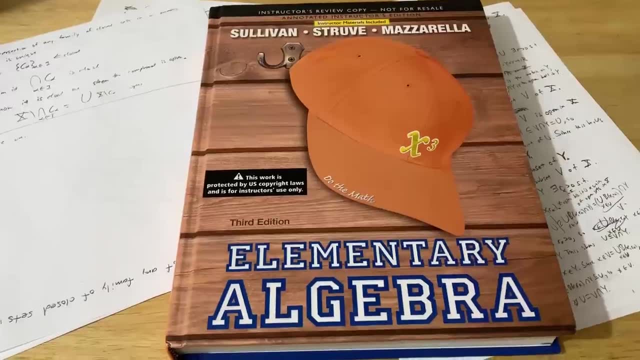 The pros of this book are that it is a great book for learning the math that's contained in it. it is widely available because it is a newer book. I'll try to leave a link in the description. The cons are that it only covers elementary algebra. it doesn't cover 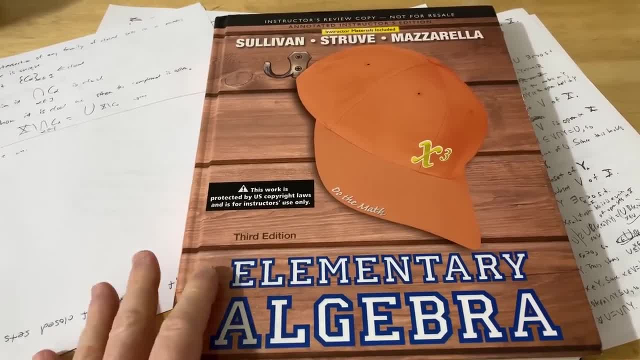 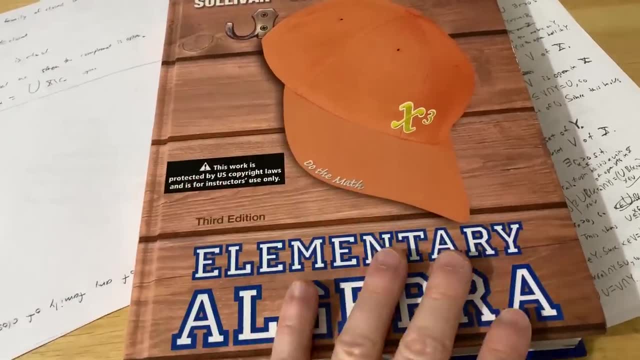 more advanced topics like trig and other topics like conics. it doesn't cover matrices, so it's not great for people who already know a lot of this math. It's going to seem very repetitious and very simple. So strictly for beginners and highly recommended for. 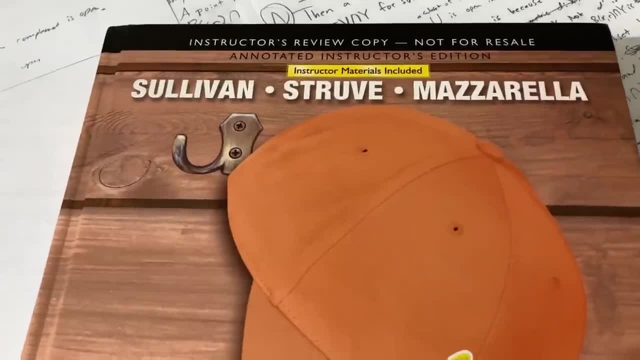 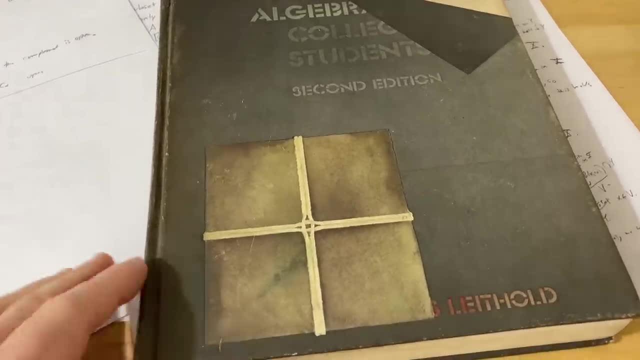 beginners. it's Elementary Algebra by Sullivan, Struve and Mozzarella. Okay, so this next book I really like This one is called Intermediate Algebra for College Students and it is by Lighthold, and I believe I said that correctly. So Lighthold is a legendary. 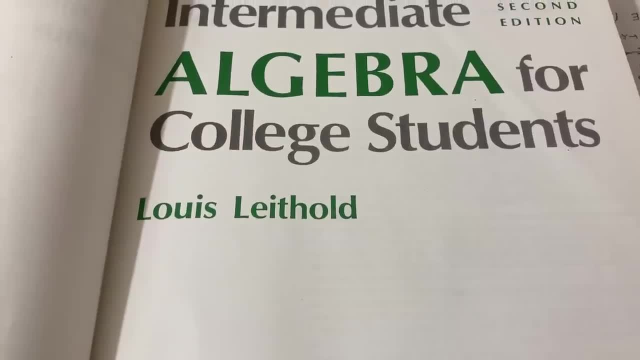 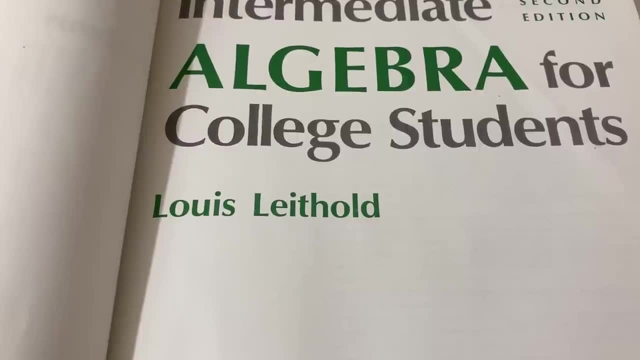 math teacher. So who is Lewis Lighthold? Well, in the 80s a movie came out. it was called Stand and Deliver and it was about a calculus teacher named Jaime Escalante who was a math professor who was absolutely incredible. Anyways, the real Jaime Escalante was inspired. 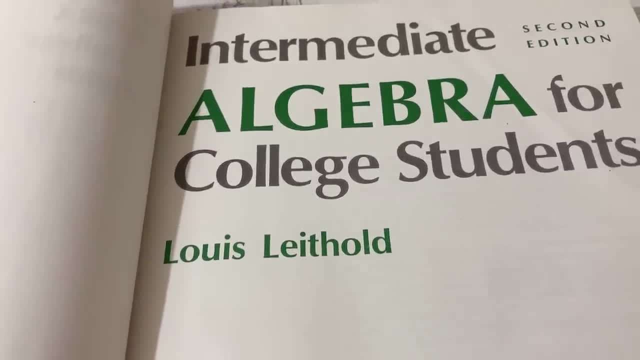 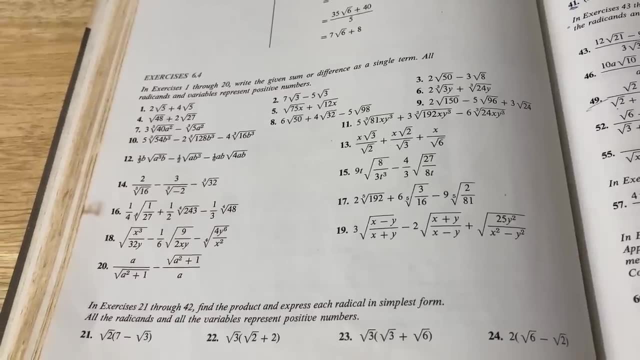 by Lewis Lighthold, and he was a legendary teacher in his time. This book also has tons of exercises, and it has answers to the odd numbered problems in the back. What I especially like about this book, though, is that some of the exercises are a little bit different. 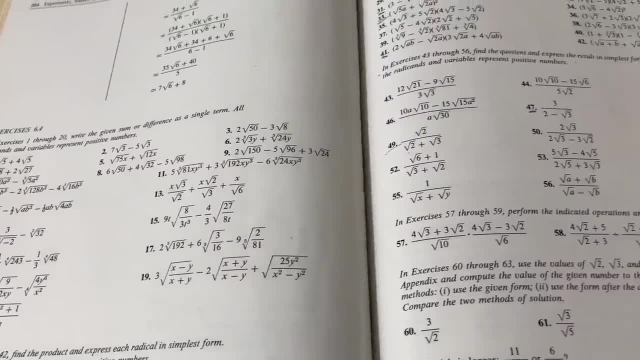 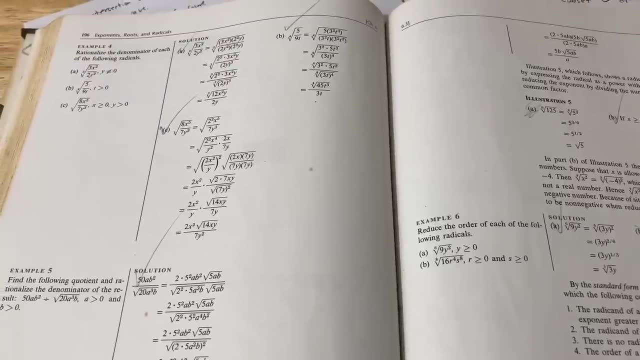 from the modern books. The other books I showed you are newer and this book is much older, so some of the exercises are different and for me that makes it a little more exciting. I've worked through tons of the examples and tons of the exercises and I think it. 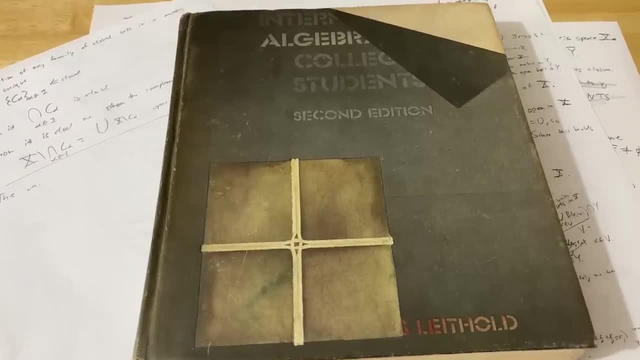 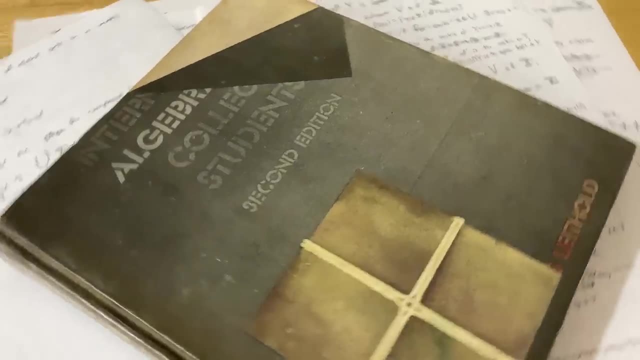 has great explanations. I really like this book. The biggest downside of this book is that it is very hard to get and if you can find it, it might be very expensive, And that's because it's out of print and it was written by Lighthold, So a very hard book to get. 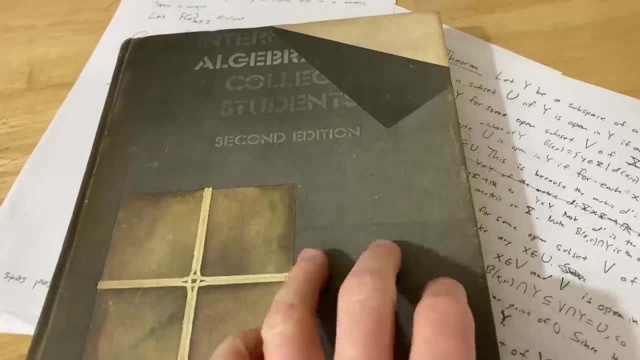 but if you can get it, I think it's worth it. My copy is really weird because it smells really weird. It has a really weird smell. I'm just going to give it a whiff. Yeah, it's got a really, really weird smell. 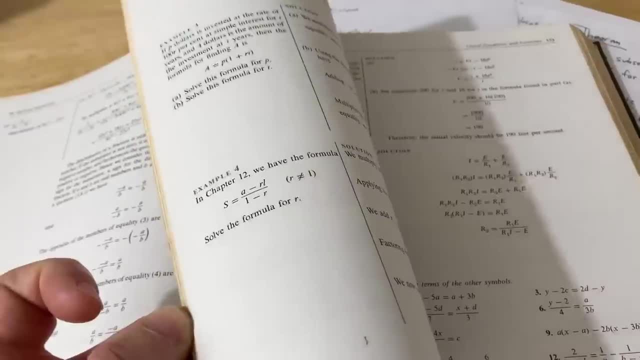 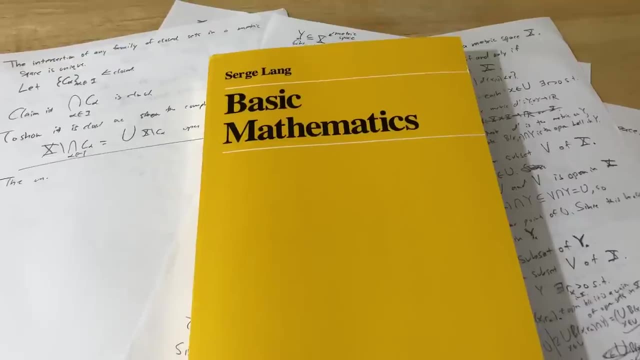 It doesn't smell like my other math books, which makes it even more mysterious. This last book is a little bit harder than the other books, even though the name is Basic Mathematics. So this book was written by the legendary Serge Laing, which is one of my. 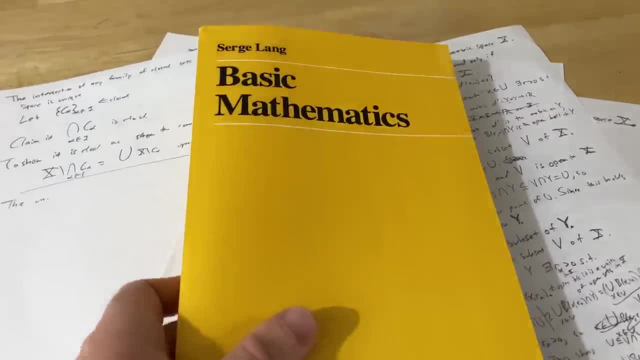 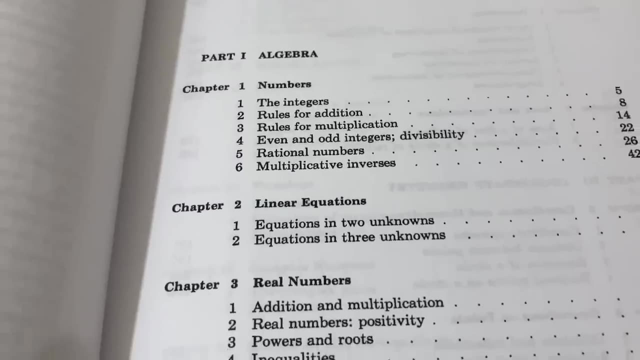 favorite authors, and this book contains basic mathematics. Let me briefly show you the contents. So he starts off with algebra, so he talks about numbers- linear equations, real numbers, quadratic equations- and then he talks a little bit about logic sets. 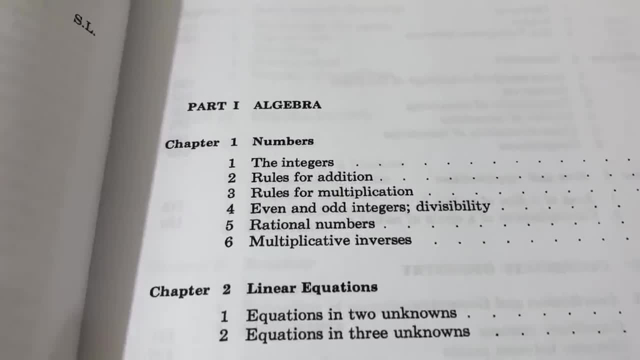 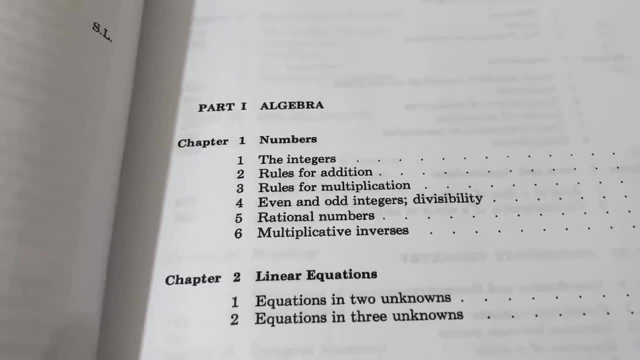 Let me just emphasize that, even though the topics might look similar to the other books, the examples and the exercises are very different. He actually has you do proofs in some of the exercises, so this is very, very different from the other books and it's way more advanced. 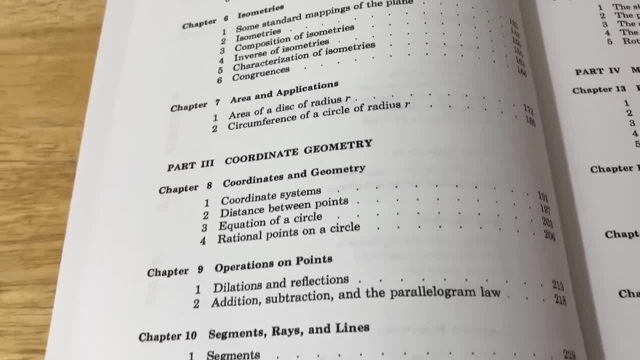 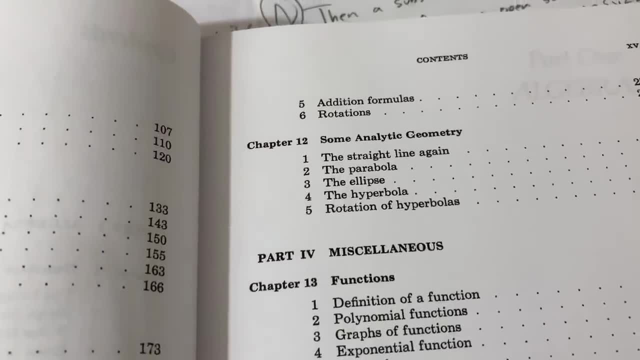 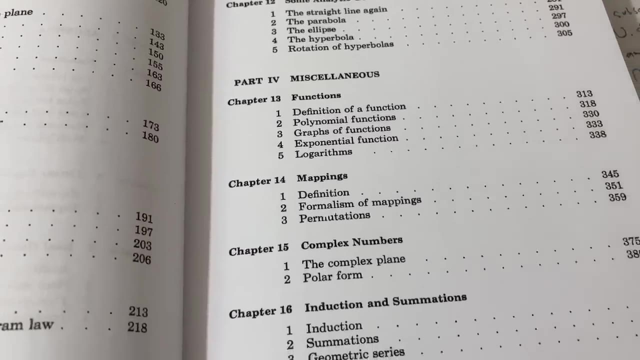 He talks about geometry, then coordinate geometry, then he goes into trigonometry. Really cool, tons of topics. He talks about some analytic geometry, so the parabola, the ellipse, the hyperbola, Functions, mappings, complex numbers, induction, determinants and there's an index- This book. 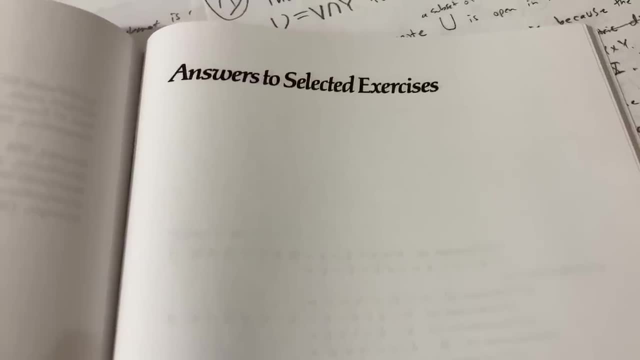 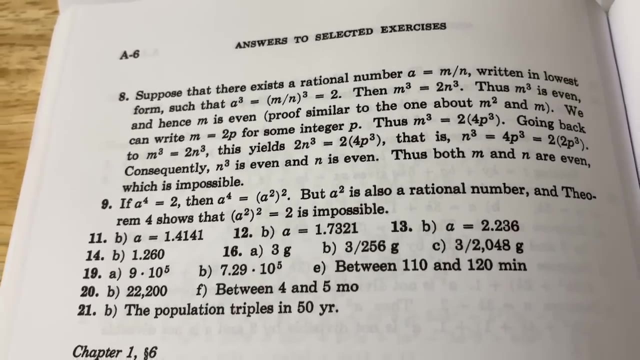 also has answers to some of the exercises, which is really really good. As you can see here, some of the answers even include solutions to the proofs. That makes it extremely useful for people who are doing self-study. This is the section where he defines the sine and 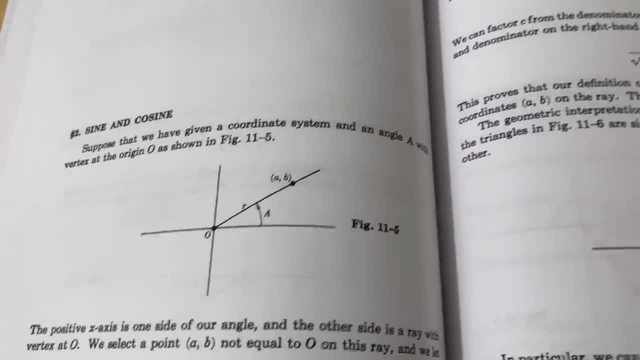 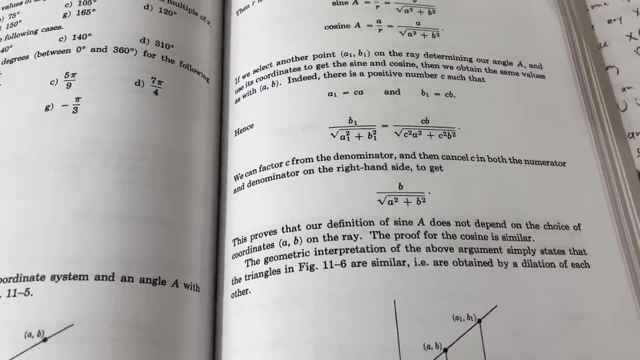 cosine function and notice how the typesetting is done. I just feel like it's extremely clean, well laid out. I really like the way that the topics are explained. This is very, very different from the other textbooks. Here are some of the exercises in one of 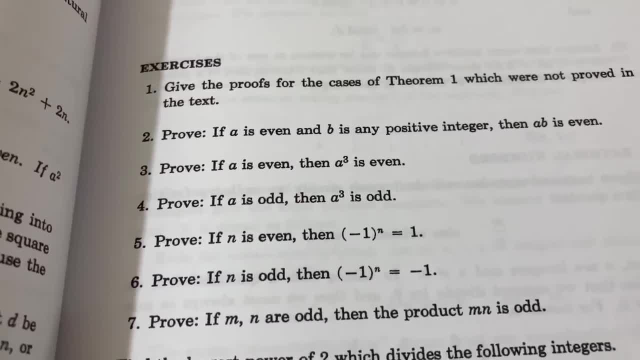 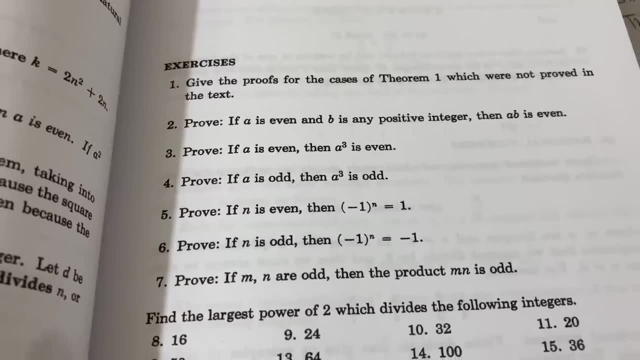 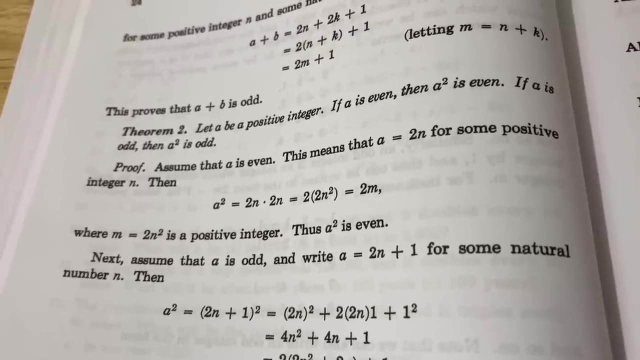 the earlier sections and notice they're actually proofs. so you're actually doing proofs in this book, which makes it a great book for self-study. and he actually has examples of proofs in the book which help you prepare for these exercises. Here's an example of one of the proofs in the book: Let A be a. 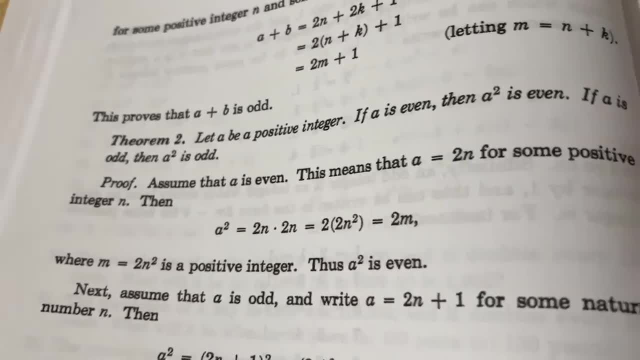 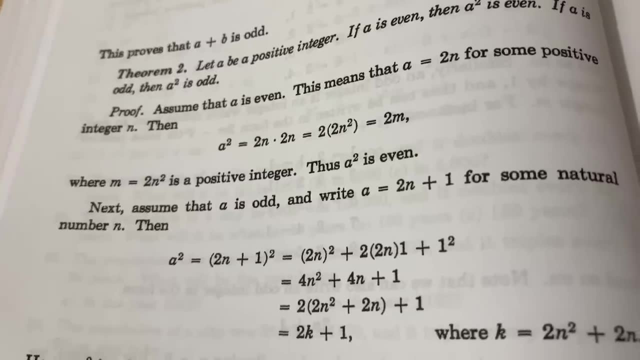 positive integer. If A is even, then A squared is even. If A is odd, then A squared is odd. And he goes through both proofs very carefully. There's no fluff and they are 100% correct. So the pros of this book are that it contains math, that 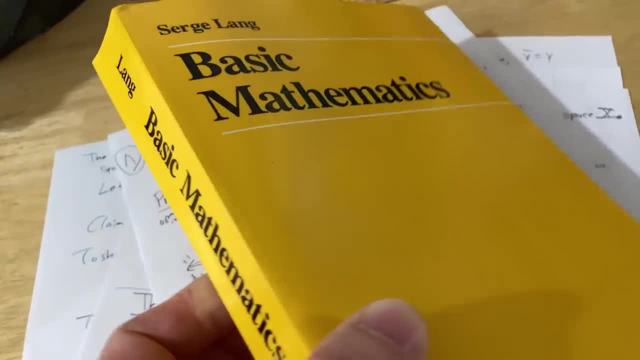 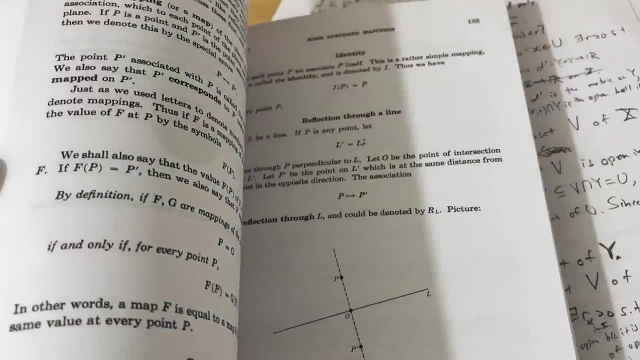 you don't see in those other books. You're gonna find math in this book that is not in the other books, and I think that makes it amazing. Another pro, I think, is that it was written by Serge Lange, who was a very famous mathematician. 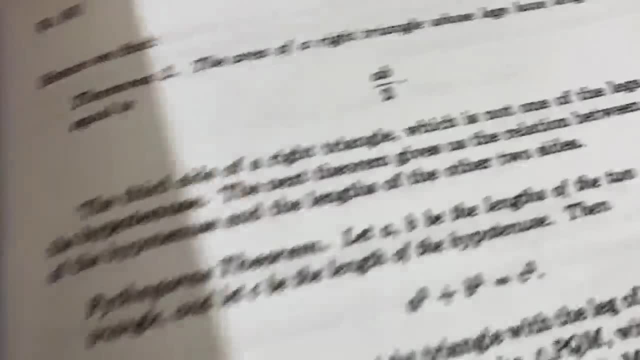 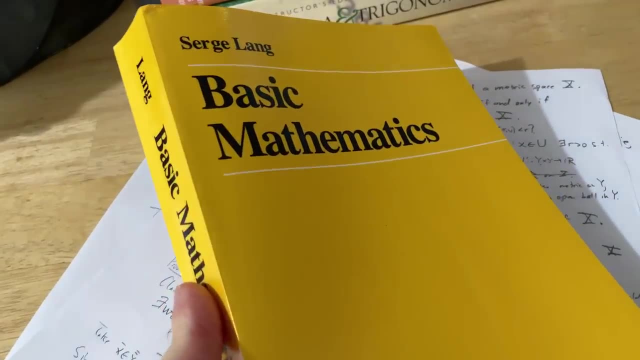 and I think the explanations are crystal clear. I'm just gonna give it a whiff. Okay, Yeah, smells pretty good. And another pro, at least for me, is the cover. I love the yellow. It just looks so cool. Now, the biggest con of this book, I think, is that 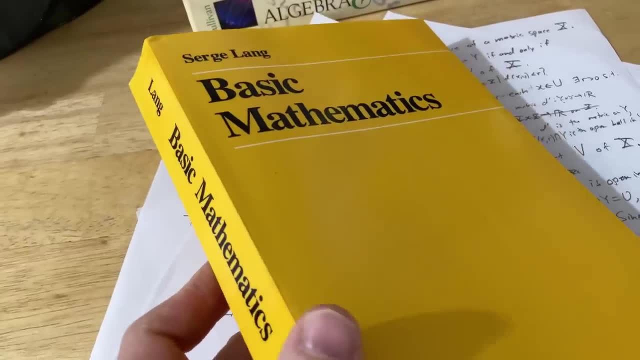 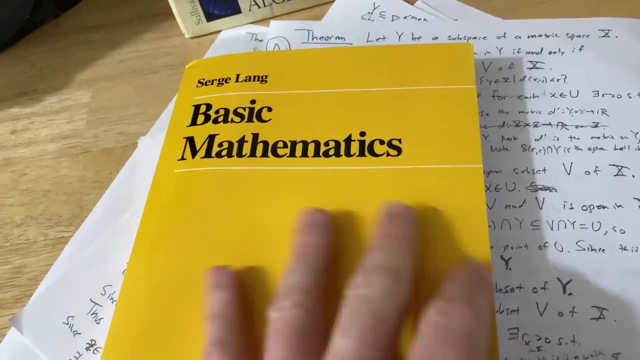 it is a paperback, and also the price. It's pretty hard to find this book really inexpensively. It actually took me years to buy this book. I have wanted this book for a very, very long time and I always decided not to buy it because 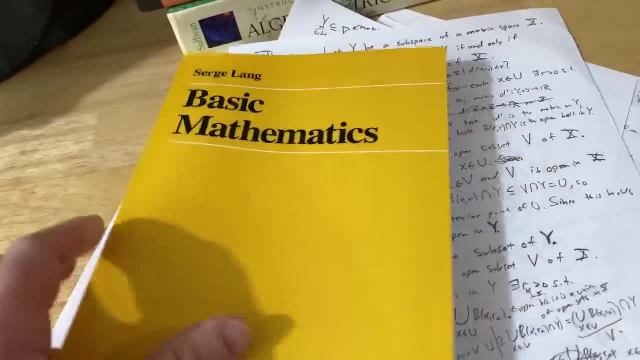 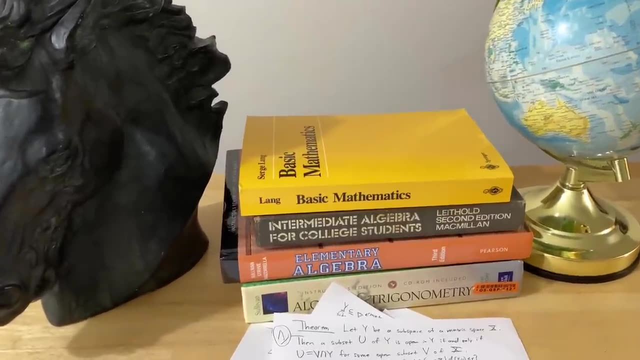 of the cost and because it was a paperback, But I'm really happy that I finally made the purchase. So those are four books For getting started with basic math And, honestly, if you have to buy one, my advice would be to buy this one. I think this is the one that's worth buying out. 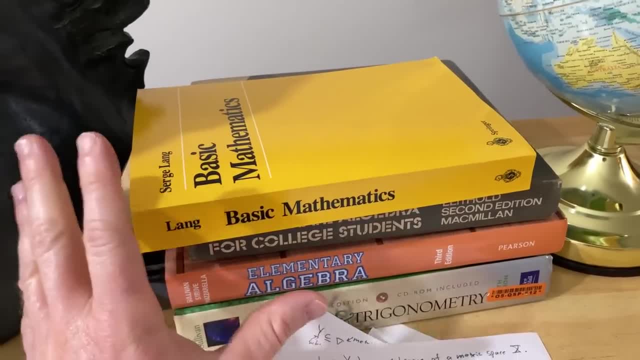 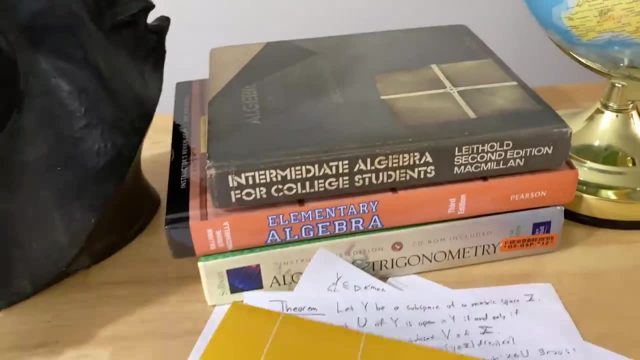 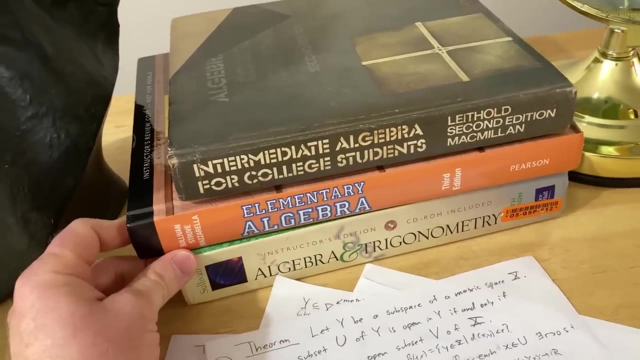 of all of these books. However, if you really really just need like a good start with basic algebra- despite me thinking that this is the best one- you're probably better off with the book by Sullivan- And if you already know some basic algebra and you want something a little more advanced, you want the other. 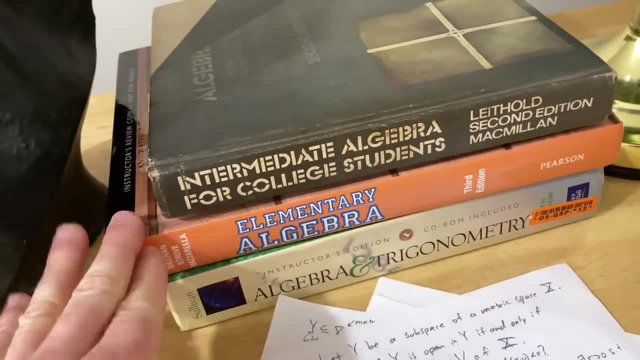 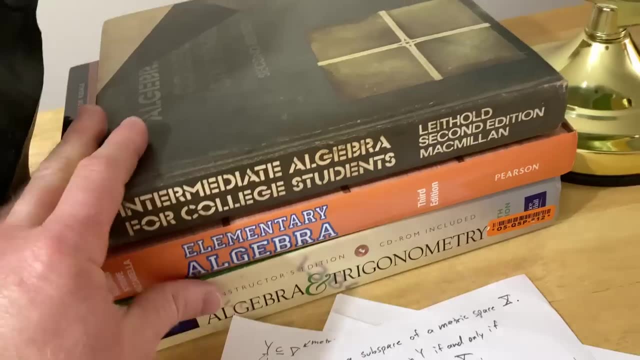 book by Sullivan, Algebra and Trigonometry. So for very, very basic beginners, go with the elementary algebra. If you already know some algebra and you want to learn trig, get this one. This one, it's pretty much- I don't want to say impossible to get. 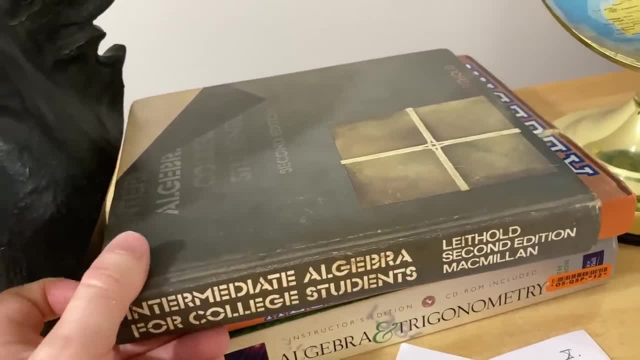 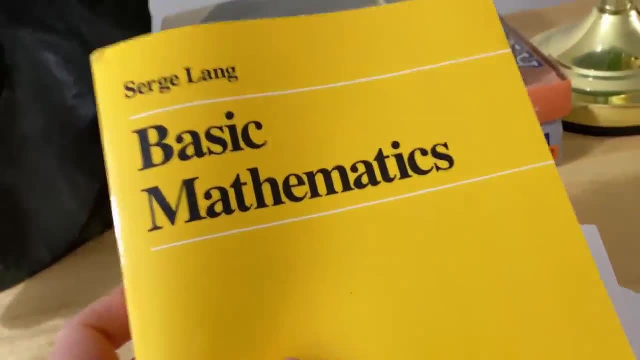 but it's just kind of hard to find right now because it's out of print, So you probably won't be able to get it, And if you want to have some fun and learn some really cool math, then I would definitely say, get this one.